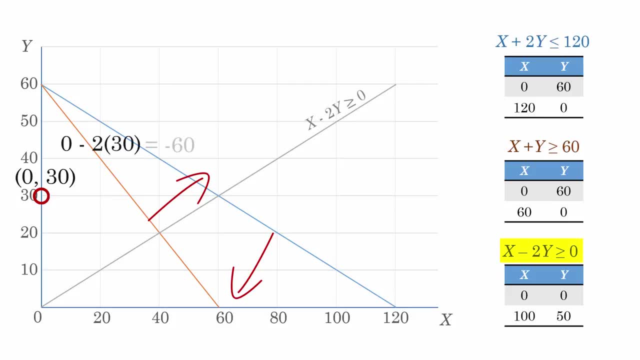 example, Putting it in the left side of the constraint gives negative 60,, which is not greater than 0. In other words, the constraint is not satisfied in that direction. Just to confirm that it is satisfied in the opposite direction, let's try this point: 40: 0.. Substituting 40: 0 gives 40 on the left side, which is: 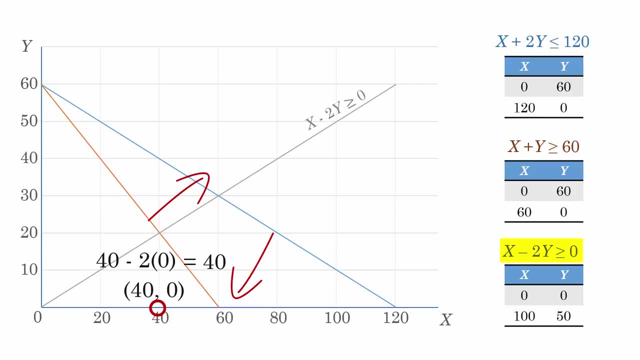 clearly greater than 0.. So the third constraint is satisfied in this direction. here, By observing the directions of the arrows, we see that the region satisfying all three constraints simultaneously is this one here which we call the feasible region. Now, the LP concept states that the optimal solution will occur at one of these corner, or 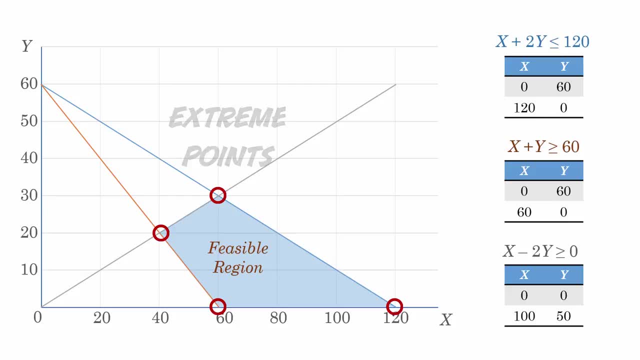 extreme points of the feasible region. It is easy to investigate all four extreme points here as they all fall on grids, but I'm just going to use the objective function or isoprofit line, Since this is a maximization problem. The objective function is to maximize z equals. 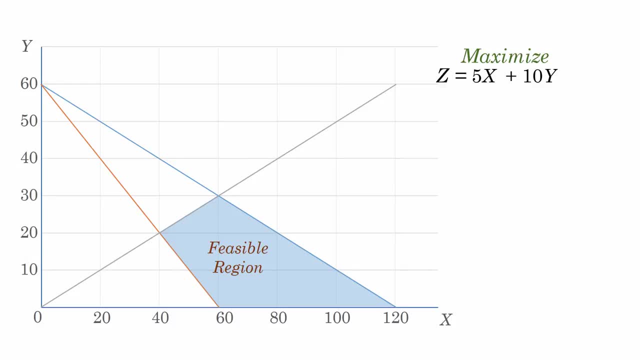 5x plus 10y. I can create an instance of a line by simply multiplying 5 and 10 here, which gives 50, and drawing the line 5x plus 10y equals 50. But that won't really display. 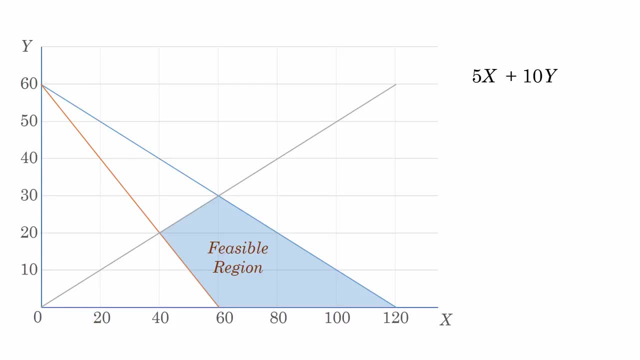 well on this graph, So I can use multiples of 50, like 100 or 200.. Let's just use 100.. So for the profit line, when x is 0,, y is 10, and when y is 0, x is 20.. Thus we have. 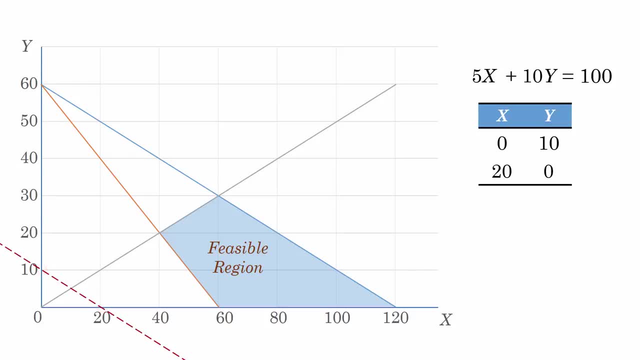 an instance of the profit line. here We now move the profit line increasingly until it touches the most extreme or corner point of the feasible region. But here we have it touching two corners simultaneously and lying entirely on a constraint line. The coordinates at the top here are easily identified to be: 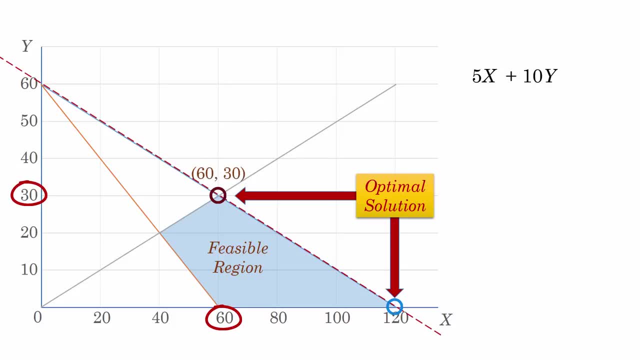 x equals 60 and y equals 30. And plugging it into the objective function gives z equals 600.. The coordinates at the corner down here are x equals 120 and y equals 0. And that also gives a z of 600.. In other words, we have alternative or multiple optimal solutions. This essentially